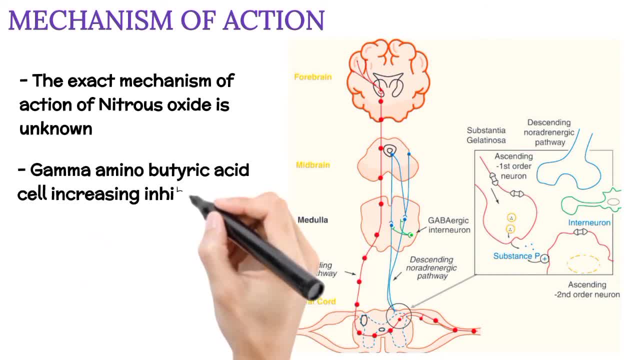 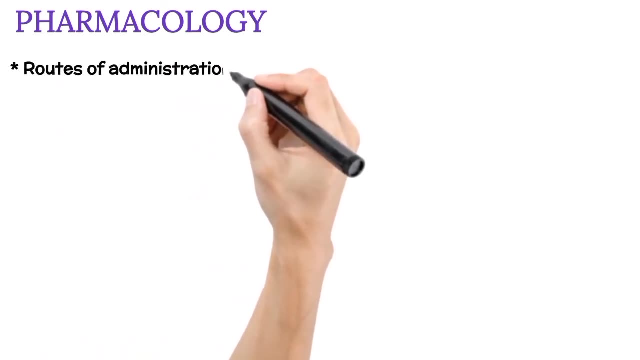 It is thought to have an effect of the gamma-amino-euteric acid cell, increasing inhibitions of the nerve cells, causing drowsiness and sleep. It moderately blocks NMDA receptors. Pharmacology: Root of administration: Inhalation Metabolism: 0.004%. 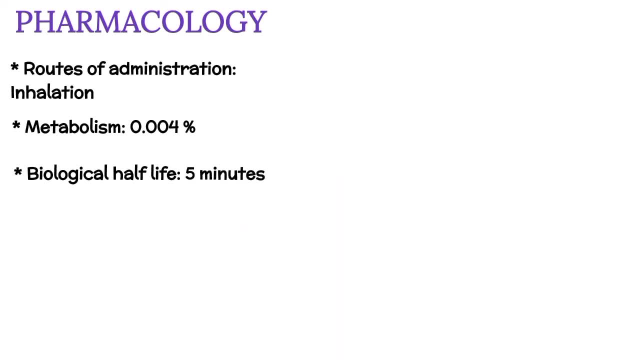 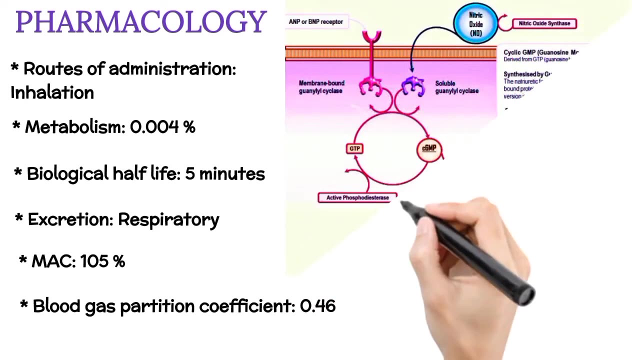 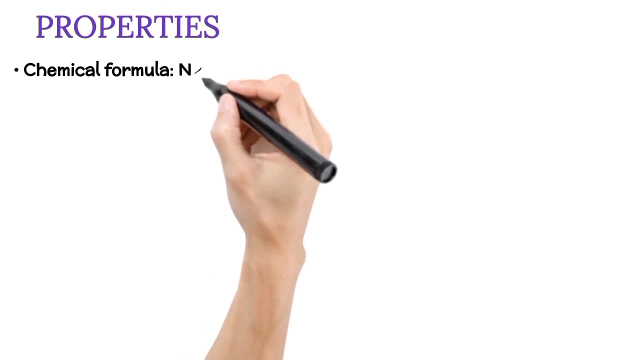 Biological half-life: 5 minutes. Excretion Respiratory: MAC: 105%. Blood gas partition coefficient: 0.46.. Properties: Chemical formula: N2O. Molar mass: 44.013 gram per mole. Appearance: Colorless gas Density. 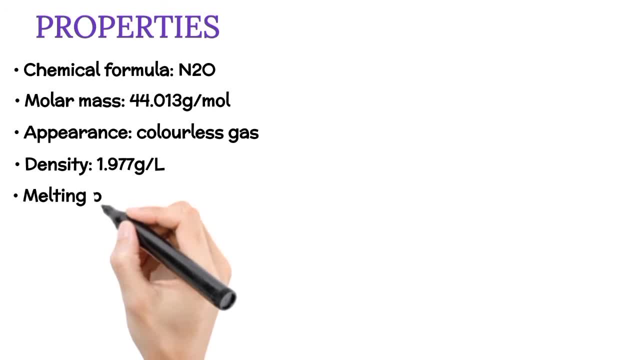 1.977 gram per liter. Melting point Minus 90.86 degree centigrade Boiling point, Minus 88.48 degree centigrade Solubility in water: 1.5 gram per liter Vapor pressure: 5150 kilopascals. 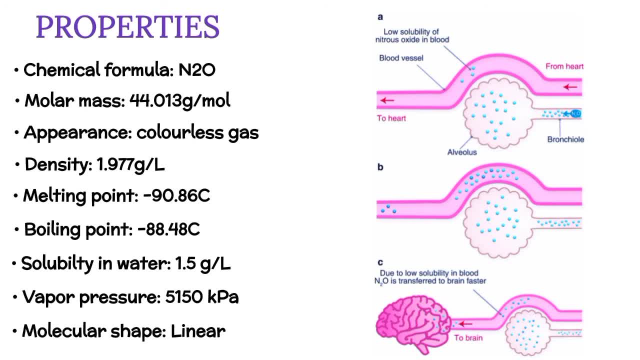 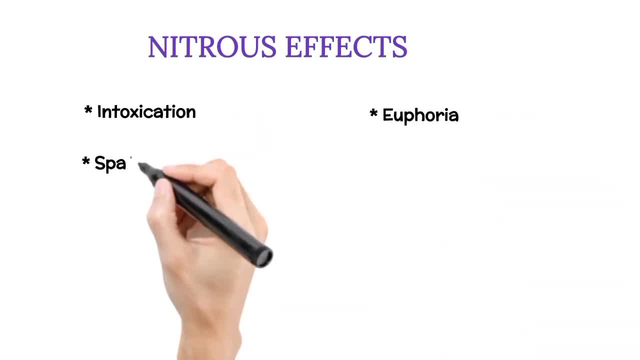 Molecular shape, Linear Nitrous effects, Intoxication, Euphoria, Spatial disorientation. Reduce pain sensitivity, Weak anesthetic, Good analgesic. It is a vasodilator causing vessels to widen. Side effects: Dizziness, Nausea, Vomiting. 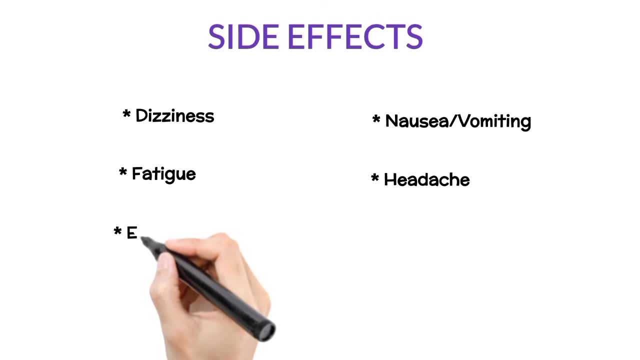 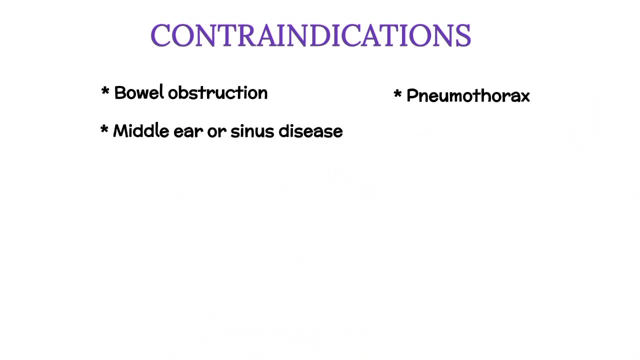 Fatigue, Headache, Excessive sweating, Shivering. Contraindications: Bowel obstruction, Pneumothorax, Metal ear or sinus disease, Scuba diving within the preceding 24 hours. Violently disturbed psychiatric patients. First two trimester of pregnancy. 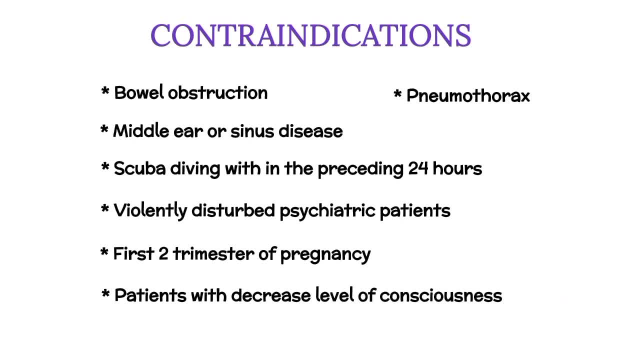 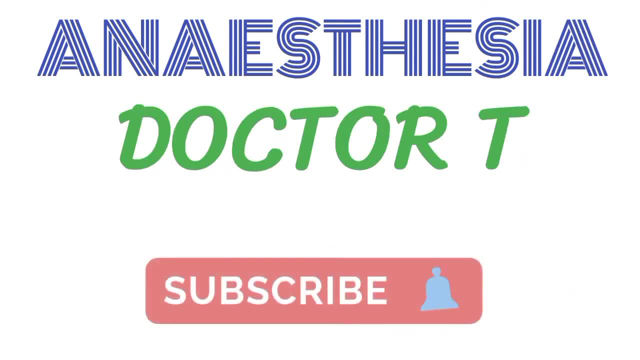 Patients with decreased level of consciousness: Anesthesia with Dr T. Please subscribe to my channel for more videos. Thanks,